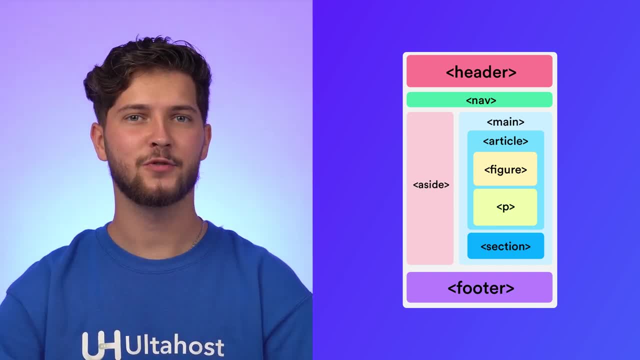 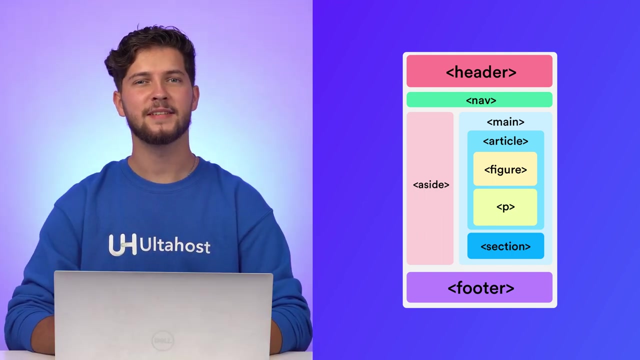 of a page or section. Nav element is used for navigation links. Main element contains the main content of the page. Article element defines content that can stand independently. Section element groups nearby content with similar themes. A side element contains less important content, often used for sidebars. Footer element is placed at the bottom. 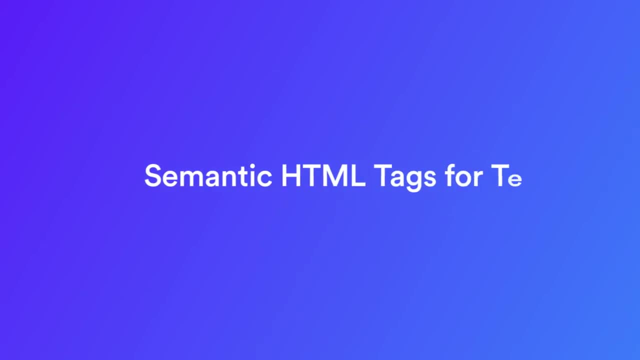 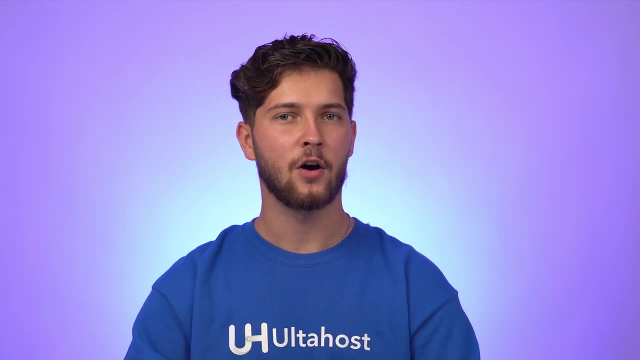 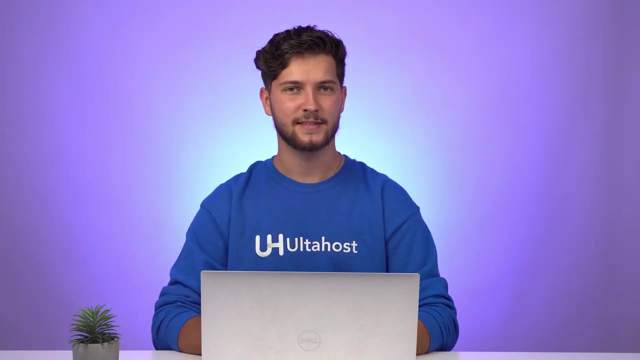 of a page for contact and copyright information. Semantic HTML tags for text. Now let's move on to the tags for written content. These tags define headings of web pages and pages with various levels of importance. H1 represents the highest level of importance. 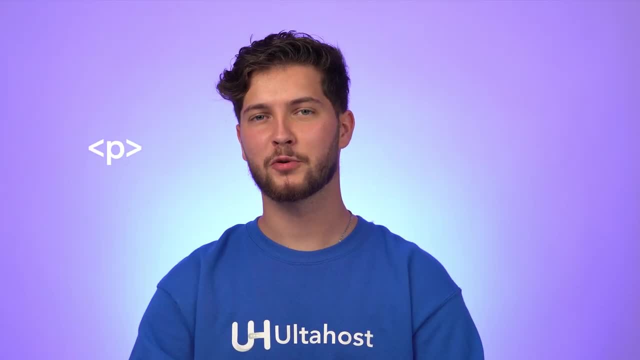 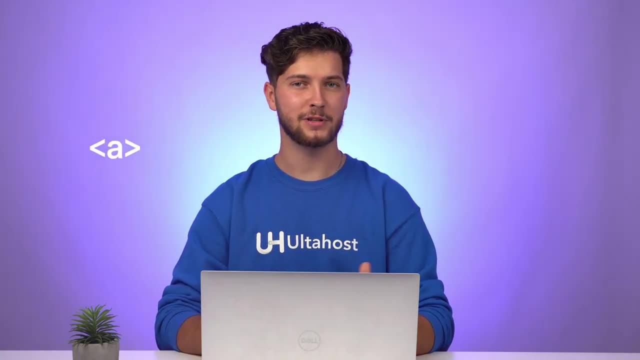 while H6 represents the lowest. The P tag represents a standalone paragraph of text. It helps structure textual content on a web page. The A tag is used for creating hyperlinks. You can use it to link to other web pages, resources or even different sections within. 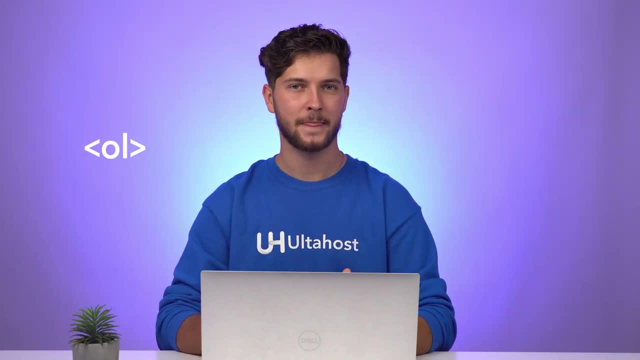 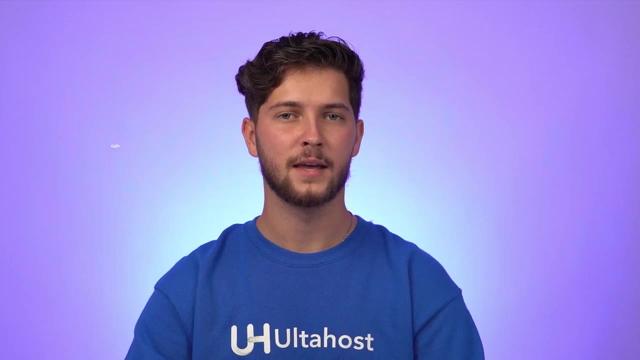 the same page. The OL tag is used to create an order list. You want to list items in a specific sequence or order, such as steps in a tutorial. The UL tag is used to create an unordered list. Unlike ordered lists, unordered lists don't have 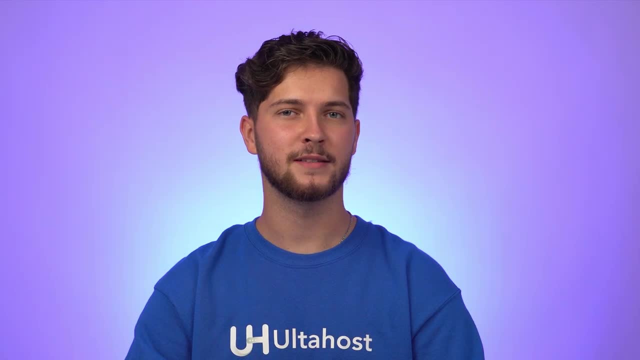 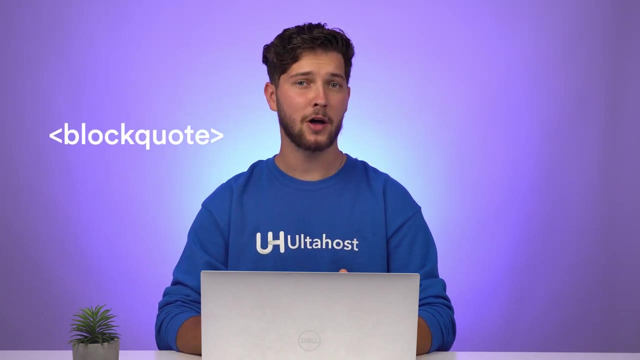 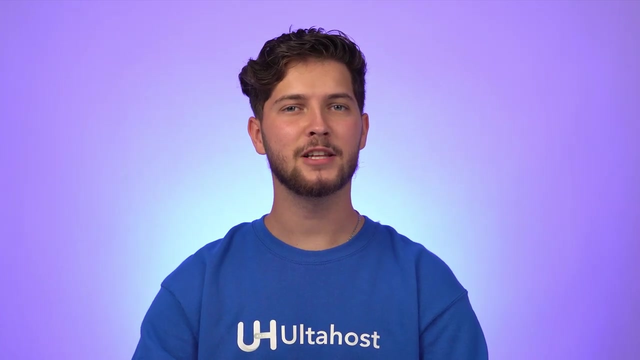 a specific sequence and items are typically represented with bullet points. These tags are used for quotations. Q is used for shorter inline quotations, while block quote is used for longer multi-line quotations. The EM tag is used for emphasizing text. It's typically rendered as italicized text and is used to give emphasis to a particular part of the content. 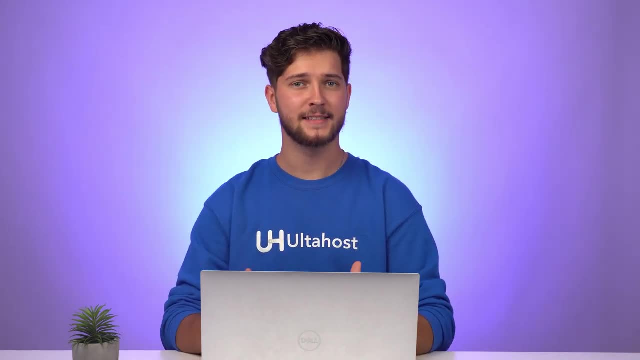 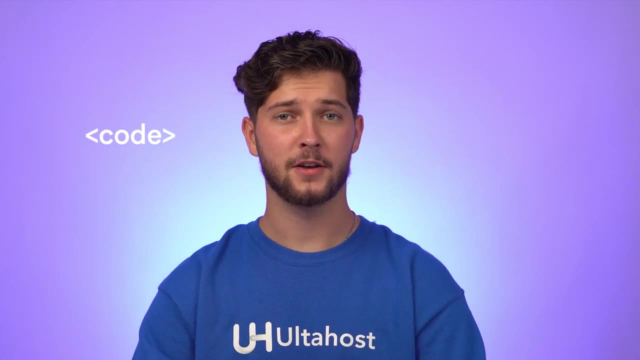 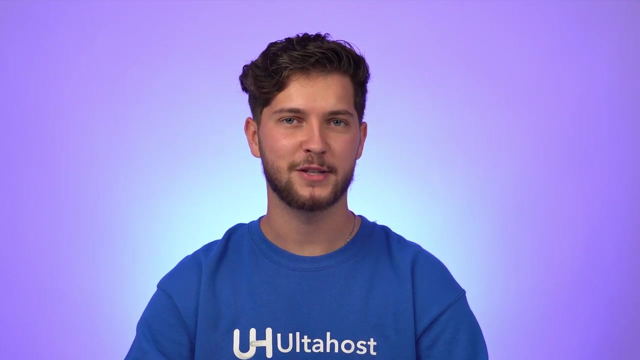 The Strong tag is used for strong emphasis. It typically renders as bold text and is used to indicate strong importance or emphasis within the content. The Code tag is used for displaying computer code. It's often used when you want to showcase code snippets within your web page. 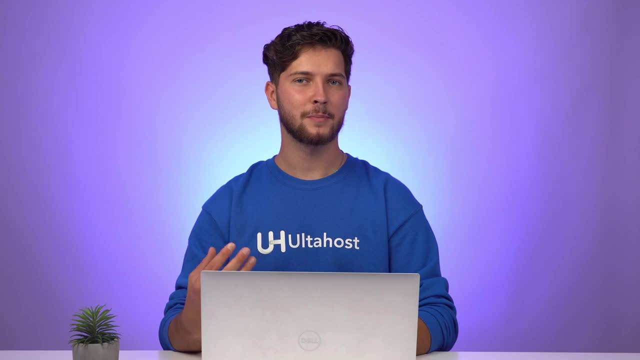 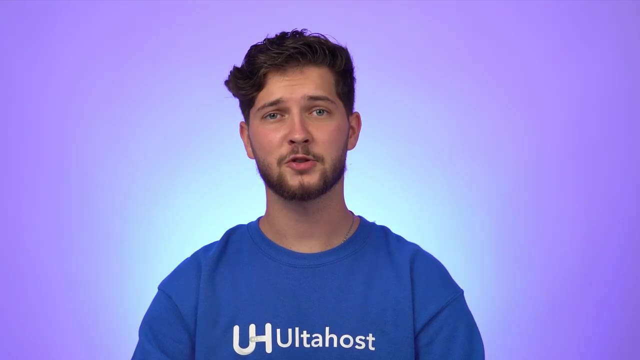 Best Practices. Before we wrap up, here are some of the best practices when using Cemented. Don't use semantic HTML tags for styling. HTML tags should not be used solely for styling. Use CSS for that purpose. Nest heading tags with semantics in mind.